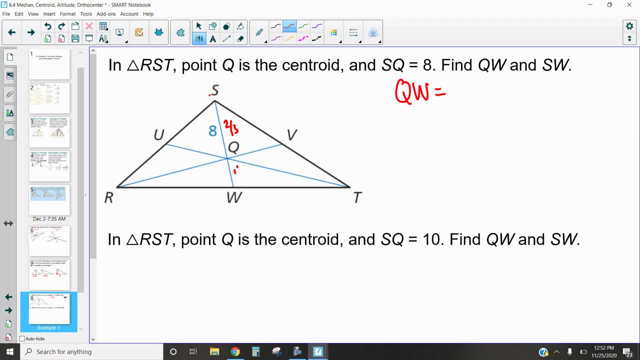 two-thirds is this and one-third- I don't know why that says one-fourth. one-third is this. That means 8 is double what the other one is. So QW is going to be half of 8, which is 4.. And then SW. 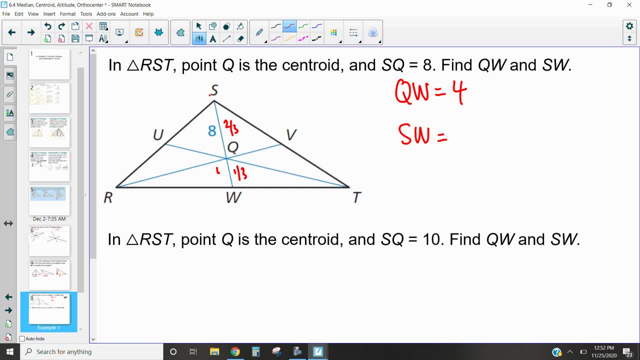 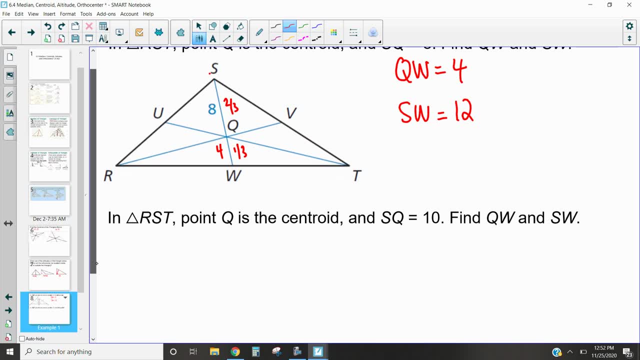 is going to be the whole thing. So SQ is 8, QW is 4, then SW is 12.. So using that two-thirds relationship or that two-to-one ratio, we can determine that distance. So let's take a look at this next example here In triangle RST. 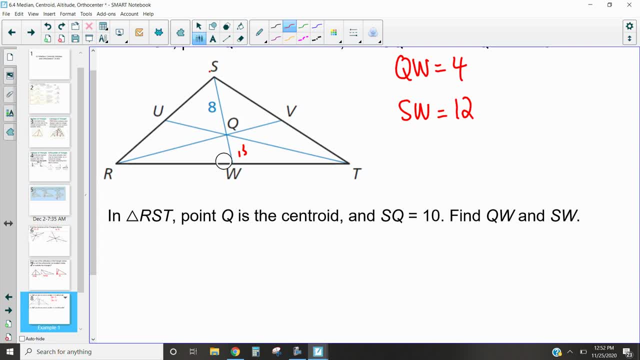 point Q is the centroid and SQ is 10.. Find QW and SW. So, again, with that being a centroid, we know that this is that two-thirds relationship to the one-third. In this case it is actually 10 instead of 8.. So, knowing that if two-thirds is 10, one-third is half of that, So that's going. 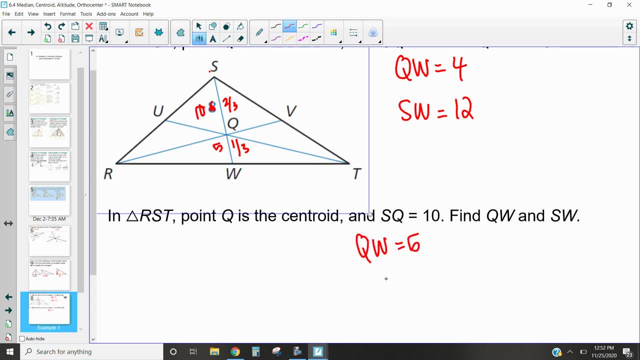 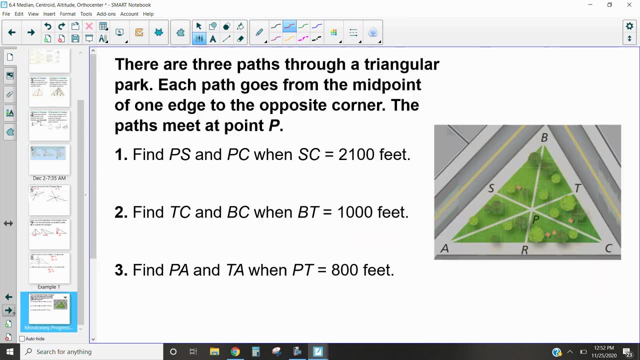 to be 5.. So we know that the length of the centroid is 10.. So we know that the length of QW is 5, and that means SW is 10 plus 5, or 15.. Awesome. Now we want to use one more. 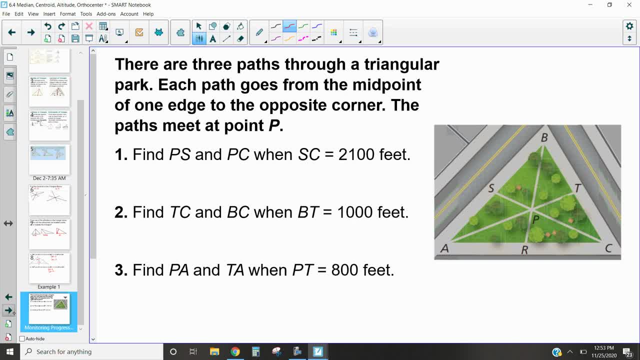 look at one more example, in which case we're using the relationships of that median and the centroid to determine what different lengths are in this problem. So there are three paths through a triangular part. Each path goes from the midpoint of one end to the opposite. 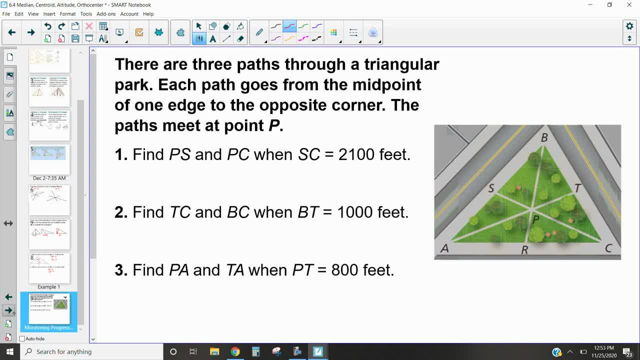 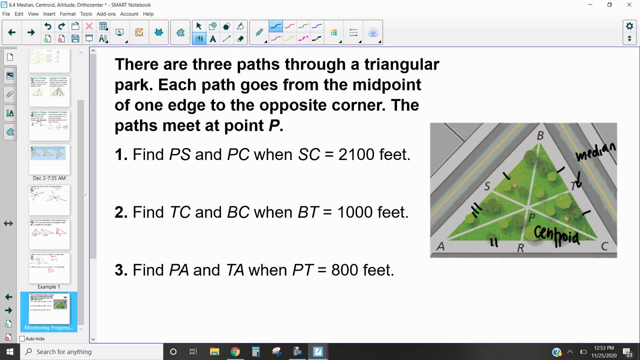 corner past me at point P. So that means, based on that definition, that this is our centroid and each of these lines here are the median. So because of that, we also know that this is the same as this, this is the same as this, and this over here is the same as the over there. Fantastic, 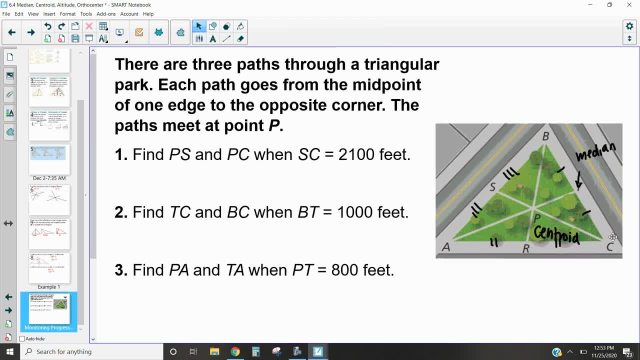 And then I'm going to shift this a tiny bit. There we go. Okay, so those are all the same. That's just what that description tells us. Now we want to find different dimensions here, So we want to find PS and PC. if SC is 2100 feet, Well, 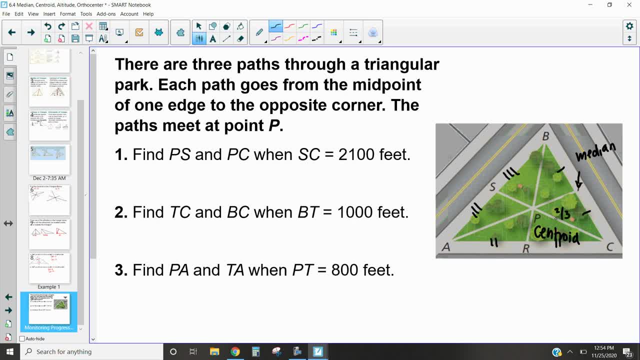 remember, if this whole thing is 2100 feet, two-thirds of it is going to be P to C and one-third of it is going to be S to P, based on that property between the centroid and the medians, So the 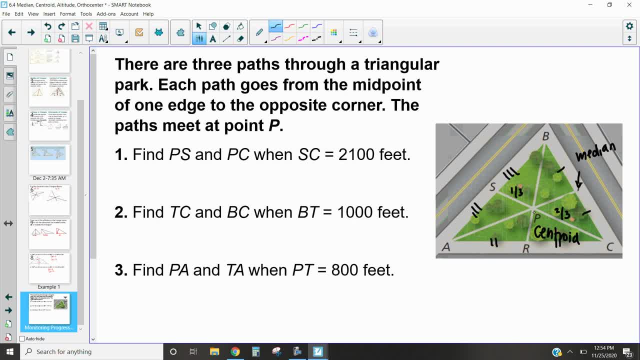 centroid to the closest vertice is two-thirds the overall distance, And so if SC is 2100, two-thirds times 2100 is going to be P. So P C equals two-thirds of 2100.. And so length, PC equals 1400. 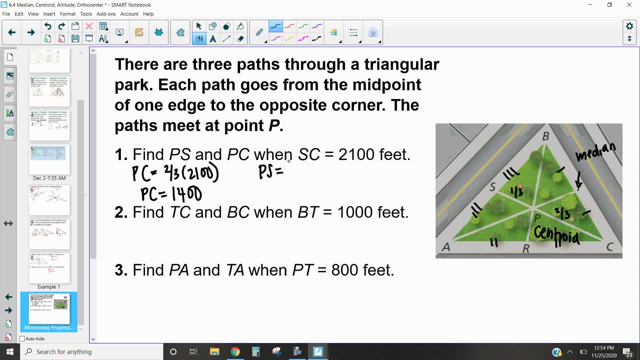 Similarly, that means that PS is going to be one-third of the distance and one-third of 2100 is going to give us a distance of 700.. Now what we want to do in this next one is find the distance, TC, which is: 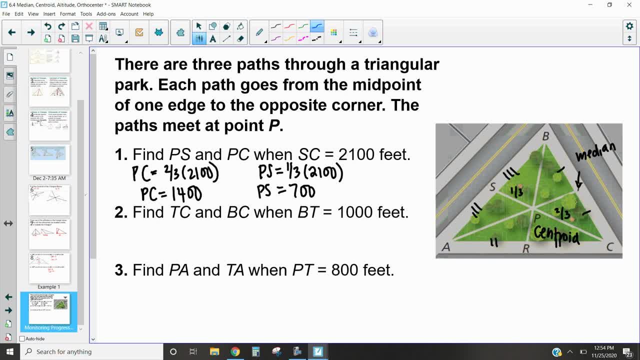 TC and B C over here. This is T. we want to find this distance twice, want to find this distance and the whole length, if we're told that this length is 1,000.. Okay so, because it's a median, that means that that side of our triangle is split into two equal. 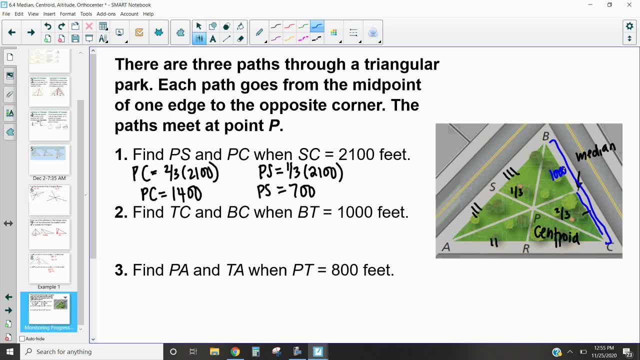 pieces. So if bt equals 1,000, that means that tc also has to equal 1,000. And if both of them equal 1,000, then that means that bc is going to equal 2,000.. Okay, lastly, we want to figure out: 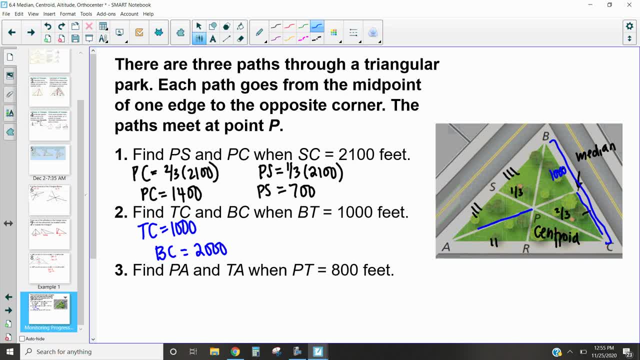 what the distance from p. we want to figure out what pa is, as well as ta, this whole long piece. if this piece here is 800.. Well, because that's our shorter distance, we know that's going to be the one-third to our two-thirds. So if that's one-third double, that is going to be p to a. 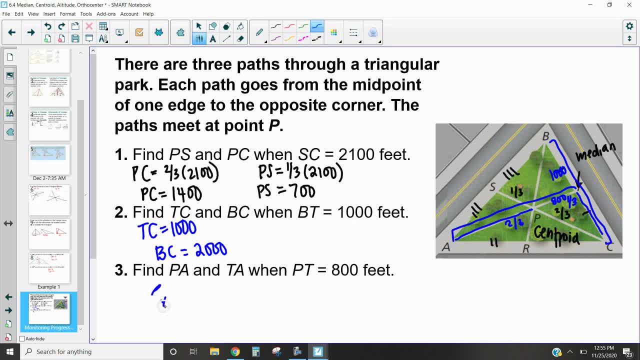 So pa is going to be- oh, not in parentheses, sorry- pa is going to be double or two times 800.. And so that tells us that length pa is going to be 1,600 feet, And then ta is going to be the sum. 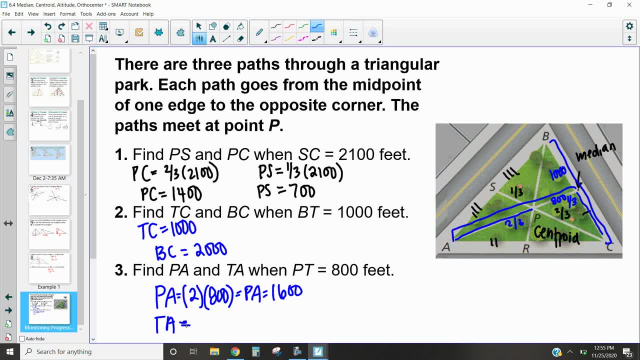 of those two things. And so if we have 1,600 feet for one length and 800 feet for the other, total we've got 2,400 feet in length. And again, all of these are in feet. And so that's how we can use the idea of a median and a centroid to determine what those distances. 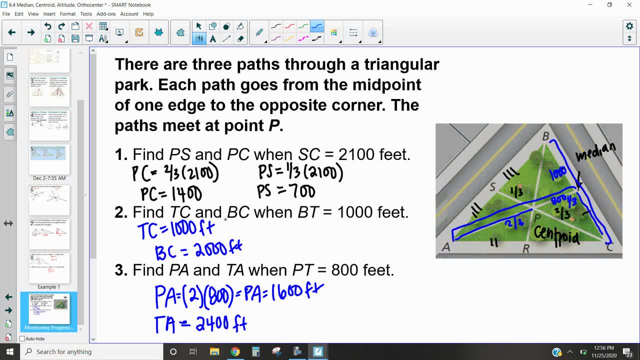 are. So what we can do is that by just knowing three things, by knowing one thing, we can figure out two other things. which is so cool about this geometry and these properties here. So if you have any questions, feel free to reach out, But that is how we can use those properties.